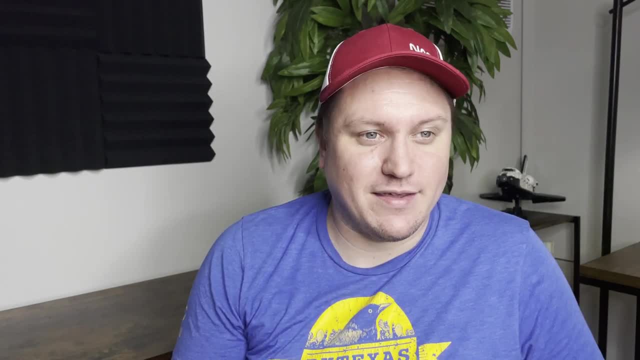 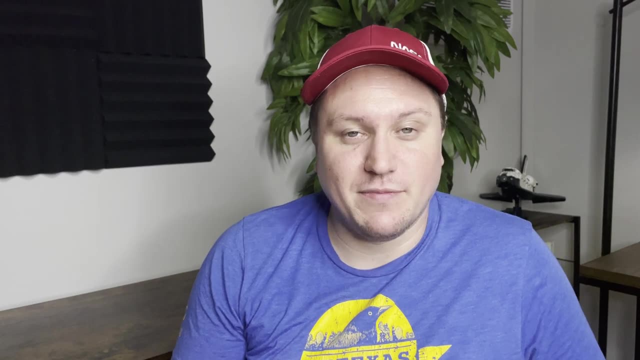 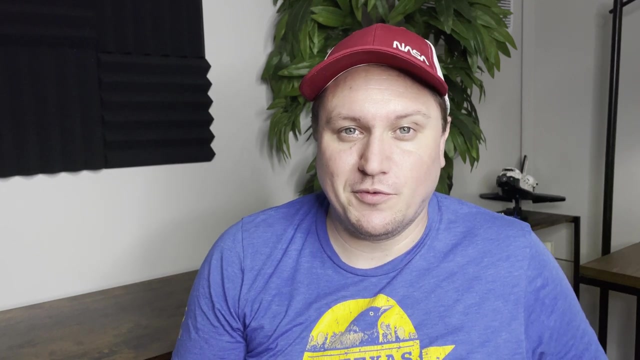 interesting study that I just read in the book called The Case of the Level Order. When I read this recently- now having made a bit of a career for the past couple of years as a writer, this was kind of shocking to me. This is a very wide range of readers and it's difficult as a writer to speak to. 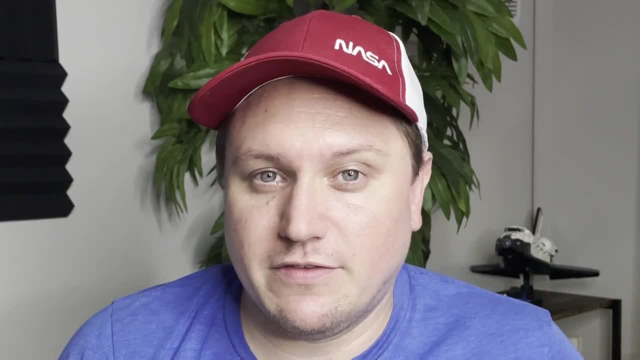 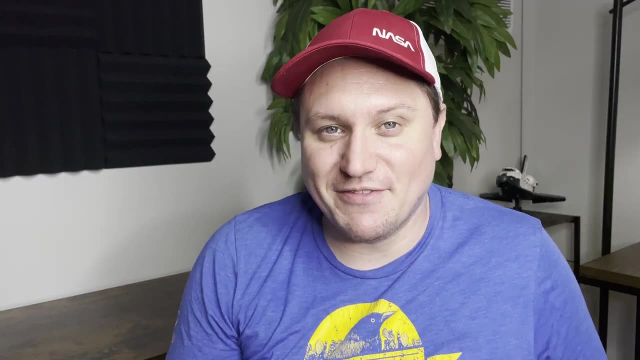 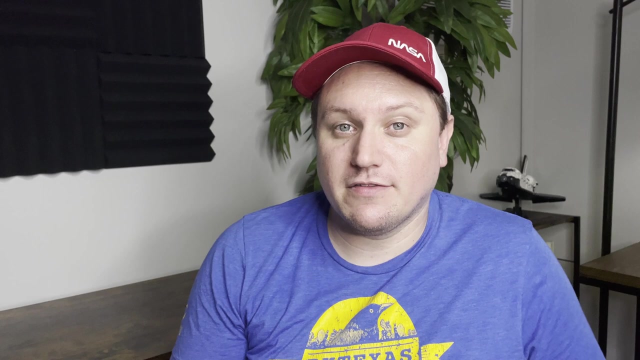 that general of an audience, And I think that Richard Trudeau does a marvelous job of achieving that goal in this book. those three categories. I really do think that you'll enjoy this book. Let's, I guess, take a quick look at some of the things that the book talks about and then I'll tell you some of my. 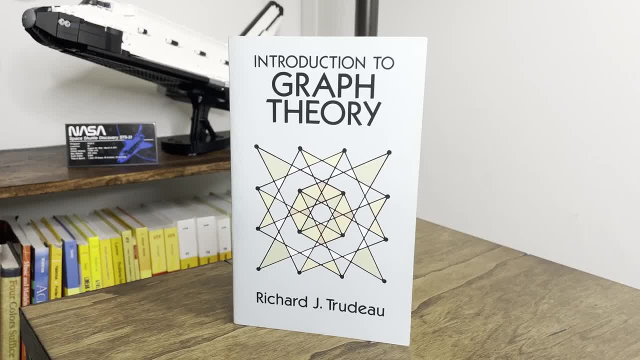 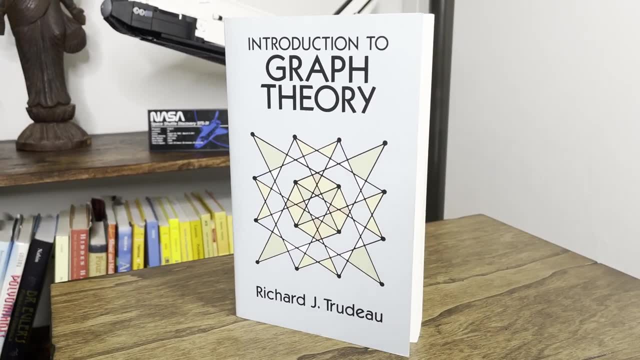 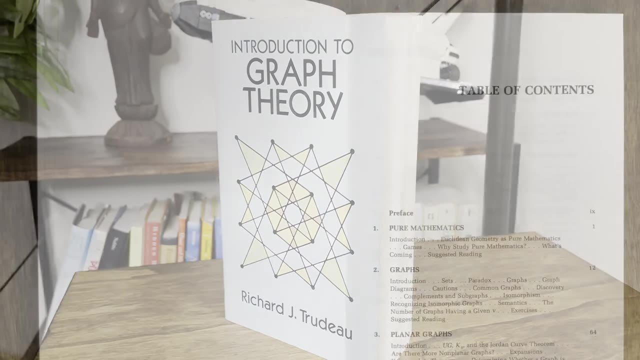 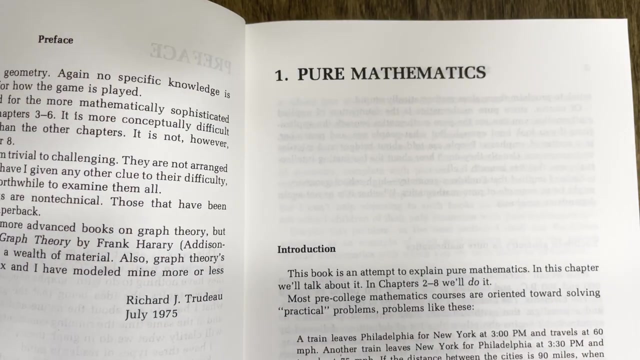 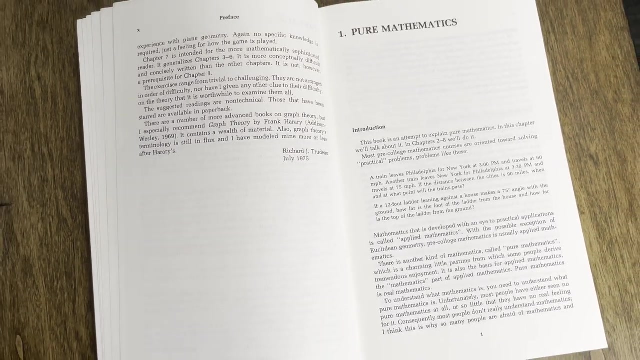 final thoughts about the book and where you can purchase it. The book starts with an introduction to pure mathematics, kind of an explanation of what pure mathematics is and why you might want to study pure mathematics, And it gives kind of an interesting analogy to a game or to games. And there's a really interesting analogy to a game. 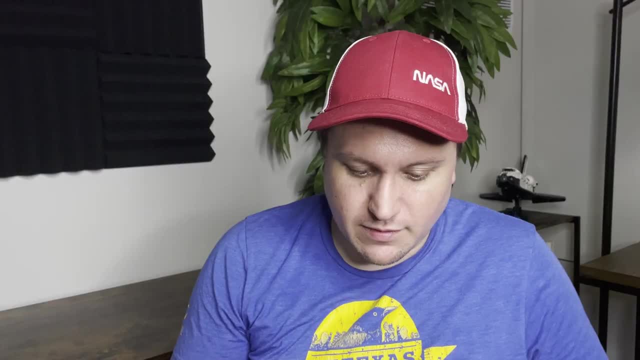 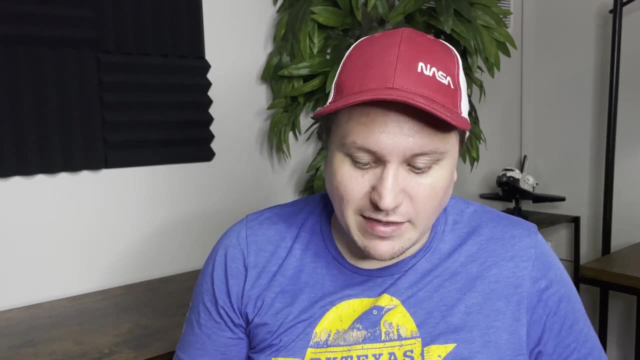 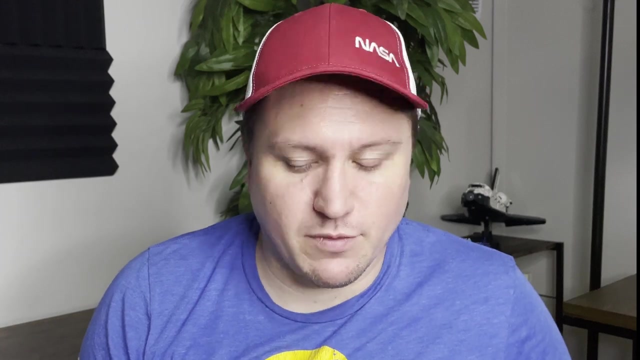 and there's a really interesting analogy to a game or to games And there's a really interesting, really nice quote in here that describes pure mathematics as basically a box of games And, at last count, it contained more than 80 of them, I believe, referencing 80 different sub-disciplines. 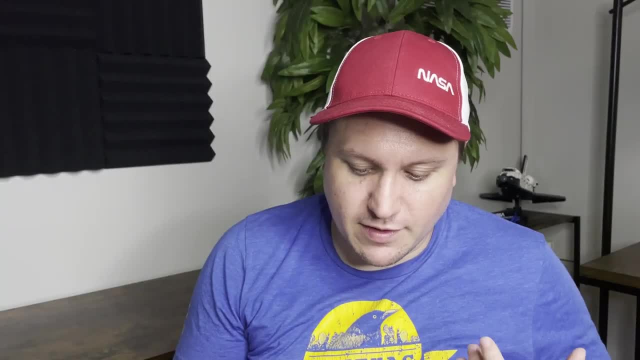 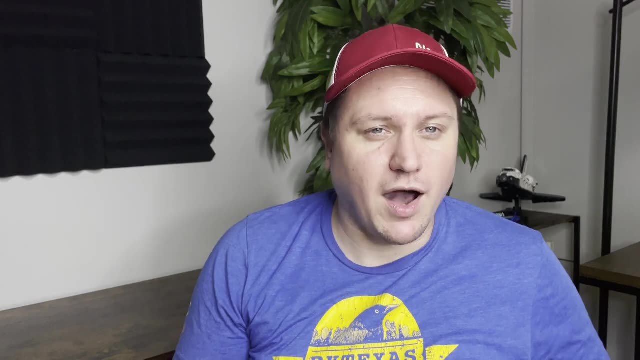 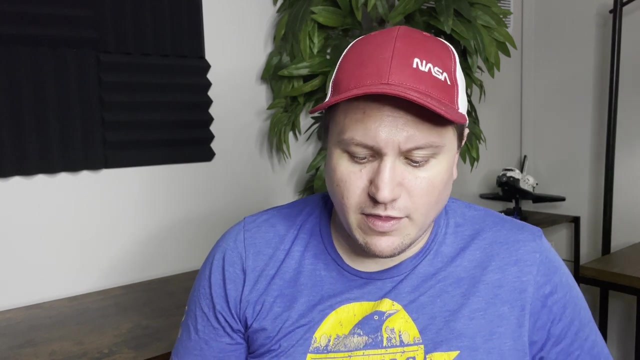 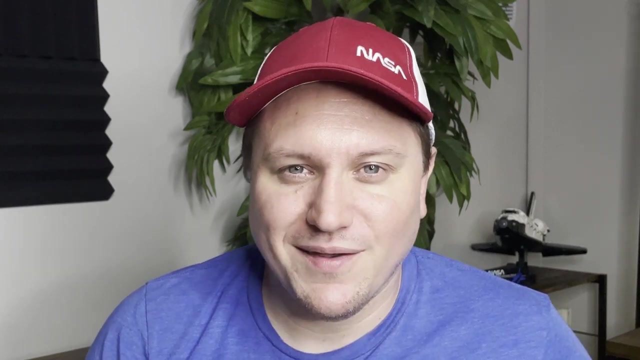 within mathematics. He gives an analogy to chess and kind of talks about how you have this game, of the game pieces and some rules for the game that you have to follow, But the board and the pieces are kind of non-essential. You could play chess with something totally different. You don't need a chess board and you don't. 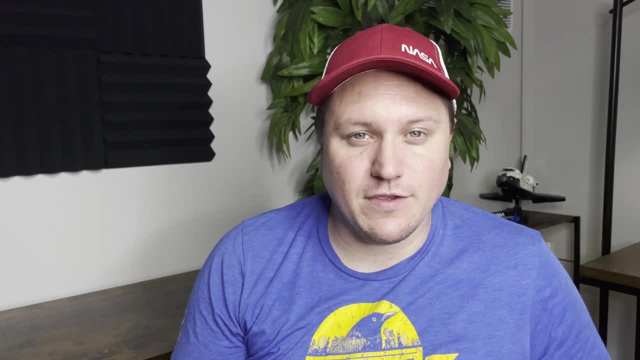 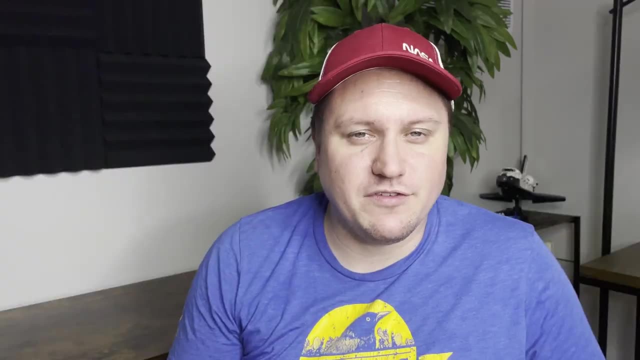 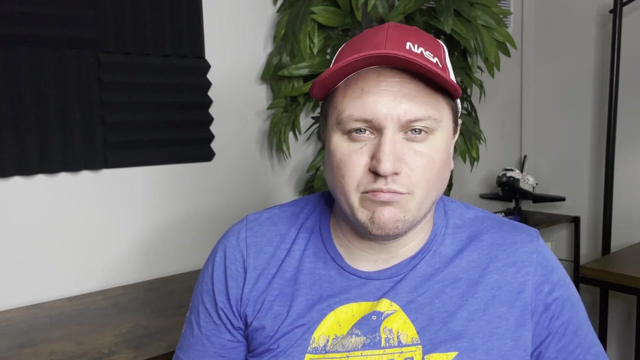 need chess pieces. As long as you have something you could consistently apply the rules of chess to, you could play chess. This is kind of true of pure mathematics, For example, in geometry you think of kind of the standard school geometry as dealing with things like points, lines and planes, And to a large extent 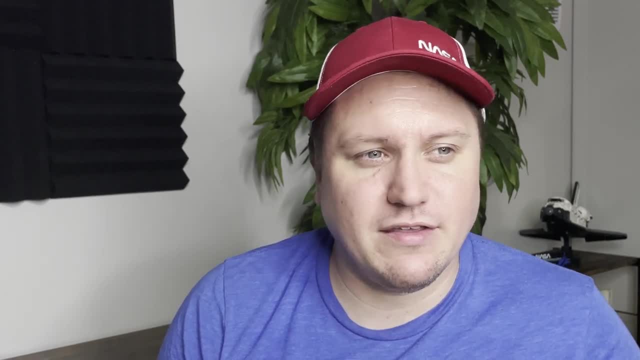 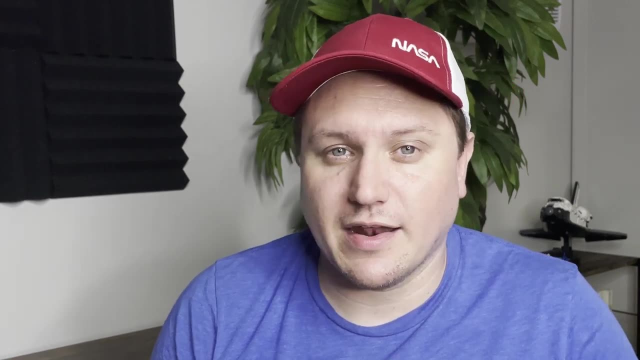 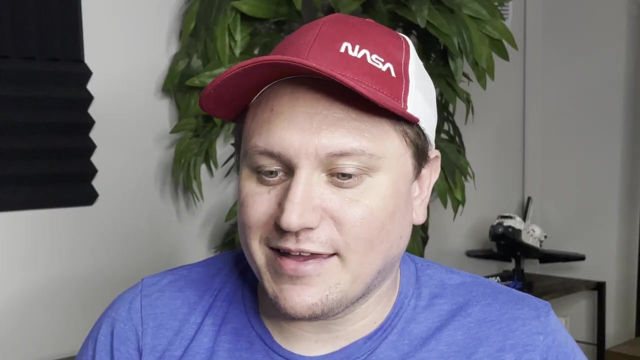 geometry is not about points, lines and planes. It's about things that meet certain definitions and things that we assume about them and then what we can do with that afterwards through the use of reason. So that's kind of a neat analogy And to some extent doing pure mathematics does kind of feel like a game. 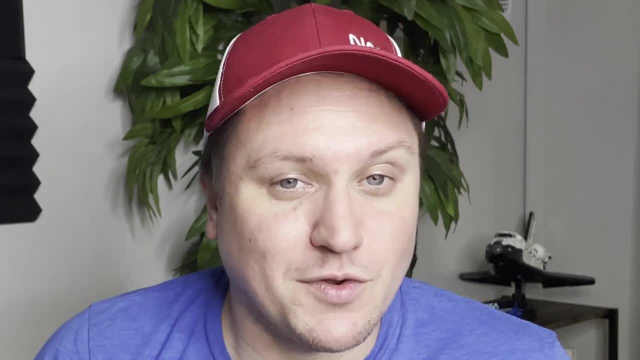 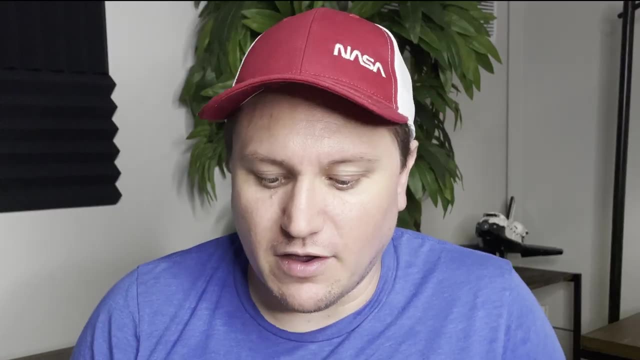 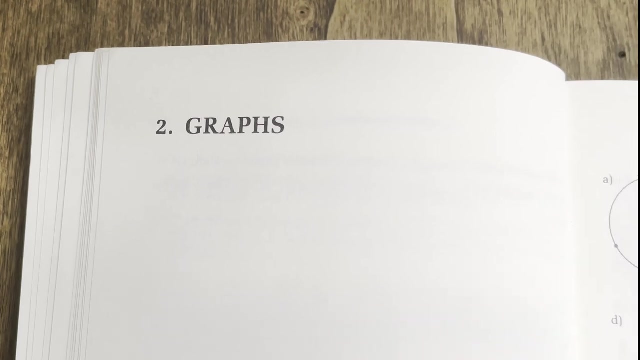 It's a game that happens to have a lot of very important real-world applications, but it does sometimes feel like a game nonetheless. After his discussion of pure mathematics, he gets into an introduction to graphs and talks about some different types of graphs and common types of graphs. 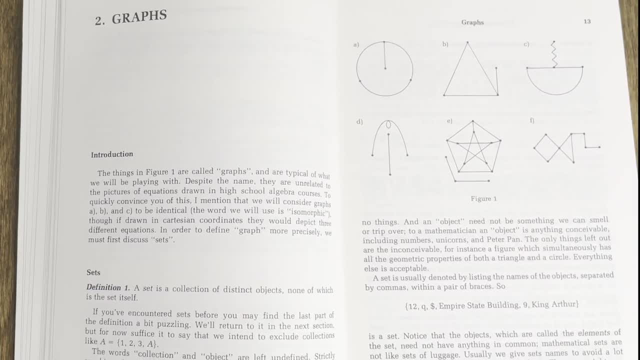 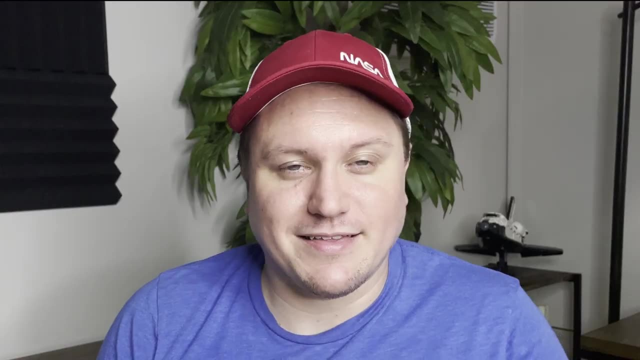 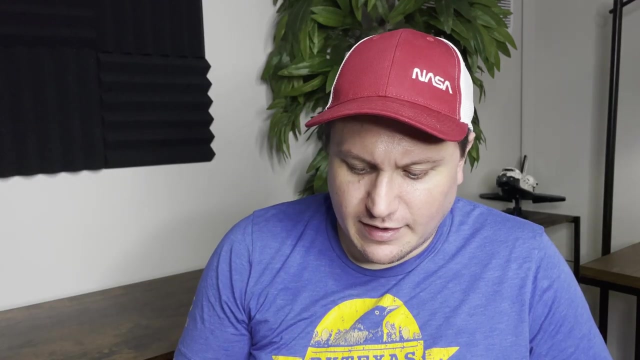 He also gets into a brief introduction to set theory and the famous Russell-Zermelo paradox, which I actually have a video about. I'll put the link to that down in the description- And some kind of basic problems concerning graphs, things like a graph isomorphism, which is a way to distinguish whether or not two graphs are the same graph. 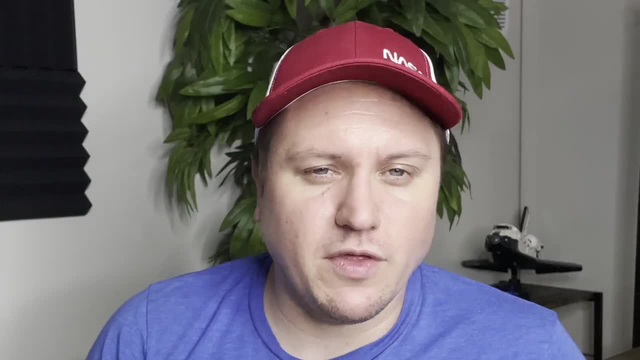 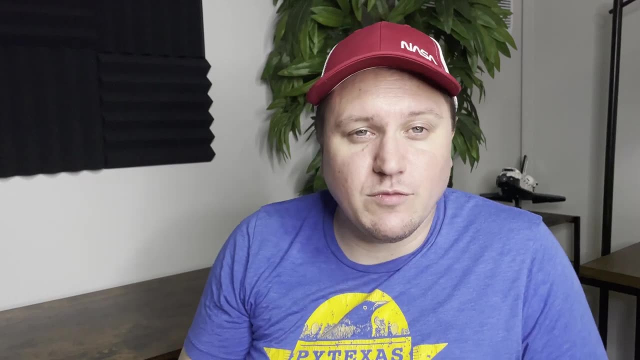 how you can recognize isomorphic graphs and a few other topics on kind of just the basics around graphs. After the introduction to graphs, he moves on to a chapter about planar graphs, which are graphs that can be drawn say like: 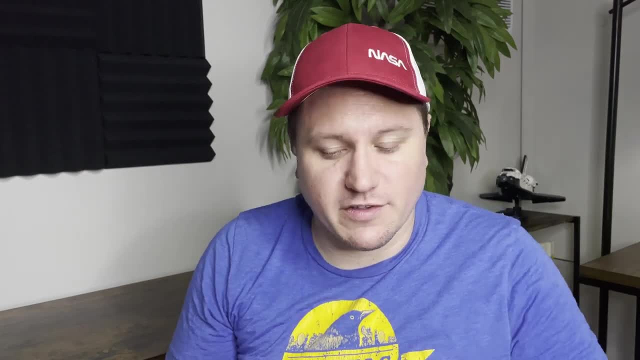 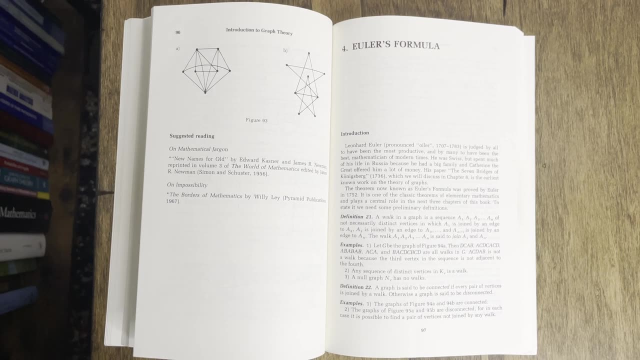 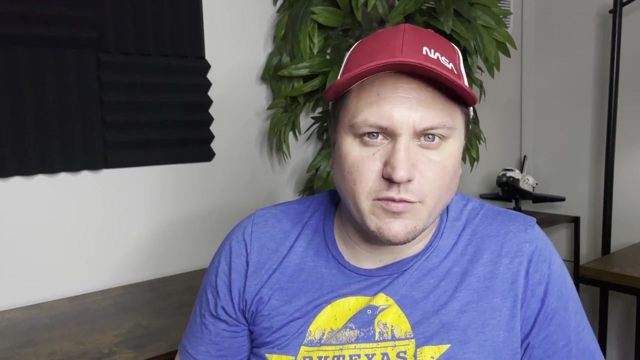 on a sheet of paper in such a way that the edges never cross each other. There's a chapter on Euler's formula, which is a famous formula about graphs. It relates the number of vertices, faces and edges in a graph in a really kind of surprising way, the first time you see it. 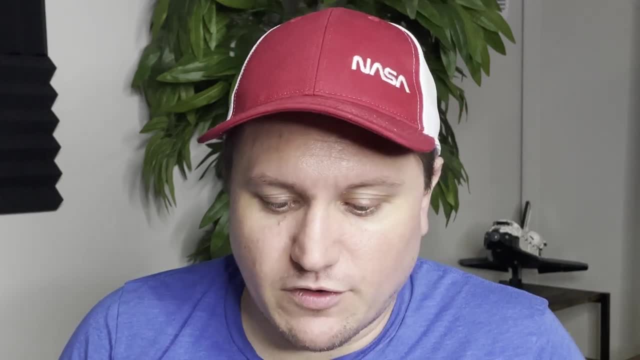 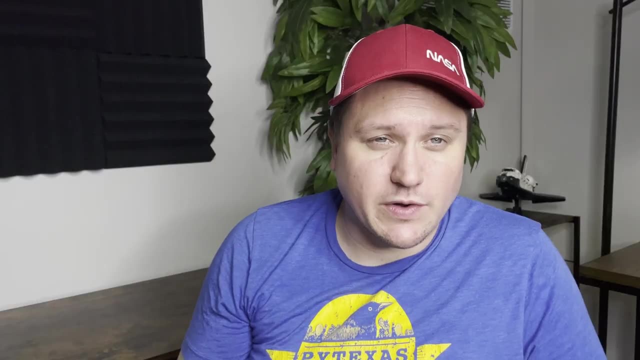 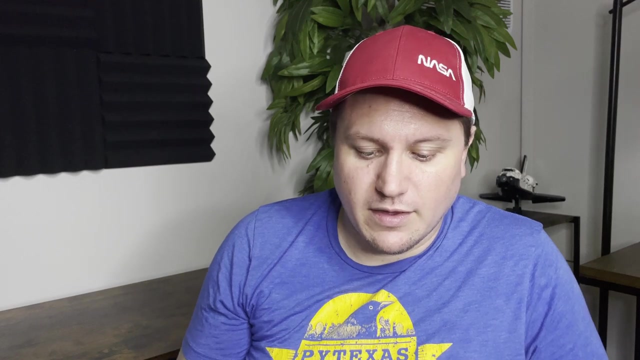 After that he talks about platonic graphs, which are graphs related to the five platonic solids. That's a really fun chapter. There's a chapter on graph coloring, which is a very famous problem in graph theory and in mathematics in general. 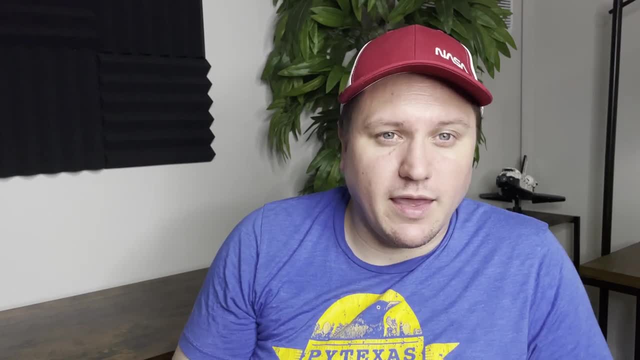 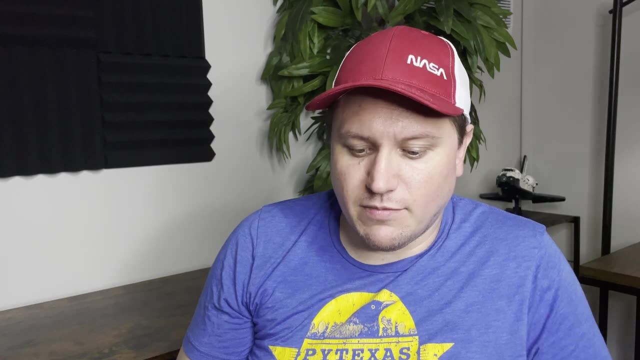 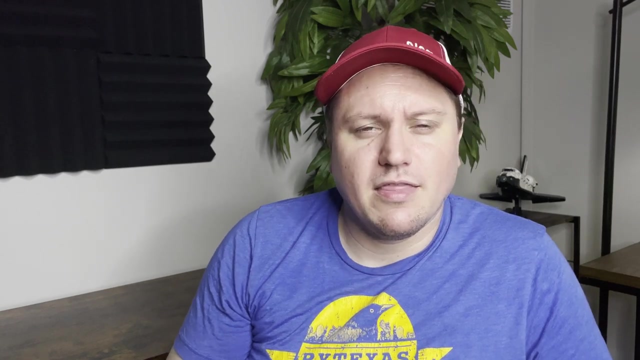 He gives a proof of something called the five color theorem and mentions what, at the time, was just a conjecture called the four color theorem. And by the time that the second or third edition- which I'm not sure which one this is, but by the time that second or third edition had been published, that proof had actually been. 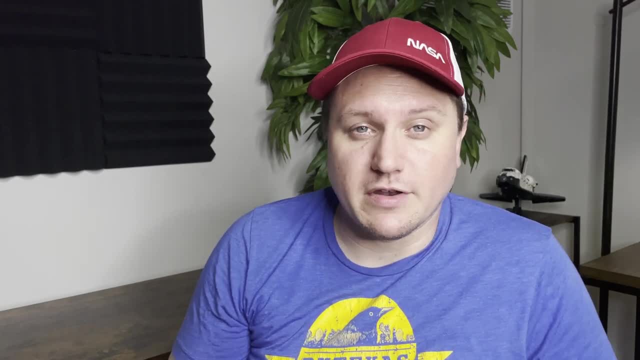 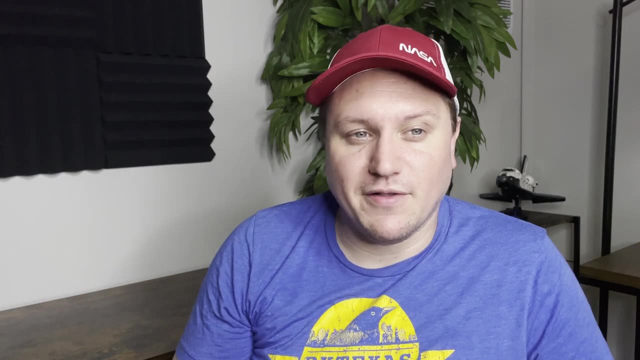 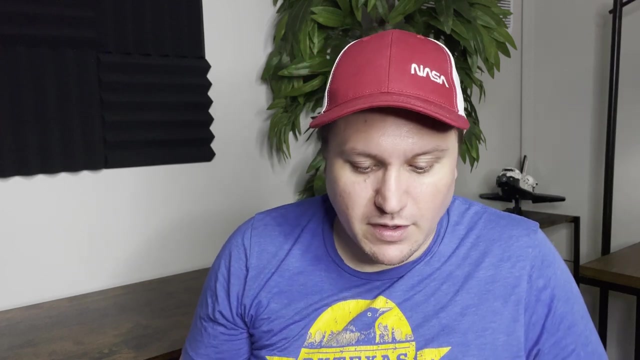 that sorry that conjecture had actually been proven And I'll do another video. I've got a great book that talks about that four color theorem in detail and gives a really great breakdown of how that works and some of the consequences and why it was important to mathematics in general. 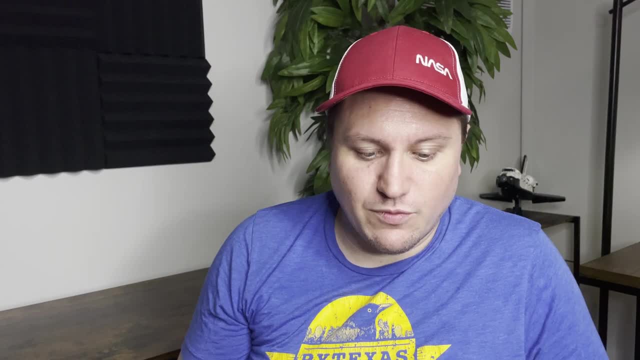 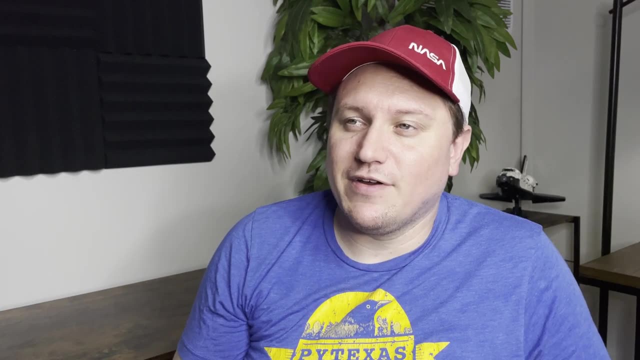 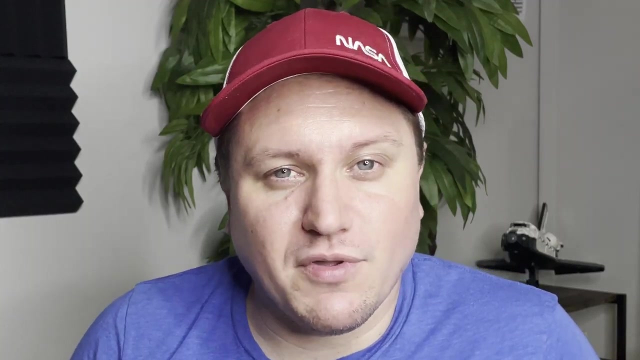 Then there's a chapter on the genus of a graph which relates graph theory to its- I don't know if you want to call it a sister discipline, but very related- topology, which we've already already mentioned. in a lot of ways Graph theory is kind of the first example of topology. 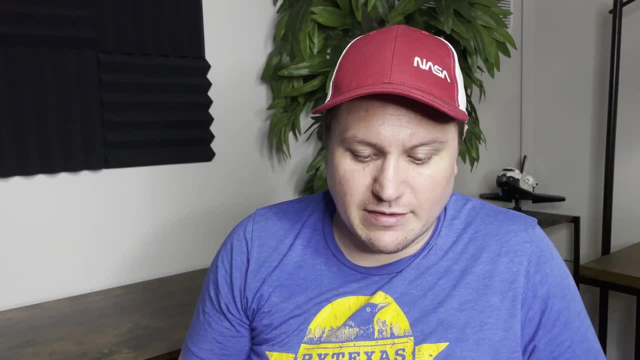 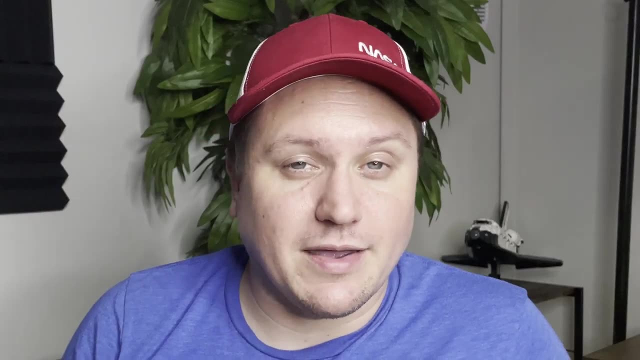 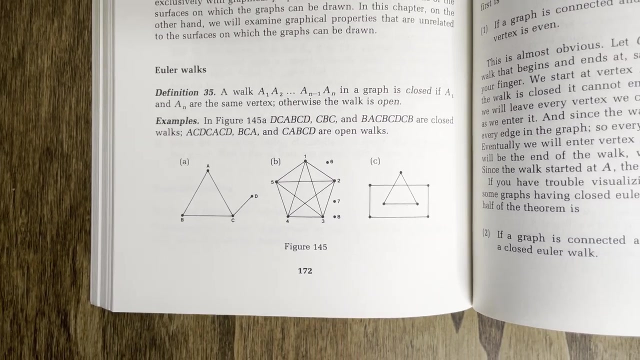 There's a big connection between those, those two disciplines, and the genus of a graph gets into and explores some of that connection between graph theory and topology. Finally, the last chapter talks about what's called Euler walks and Hamilton walks, And this goes back actually to the beginnings of graph theory. 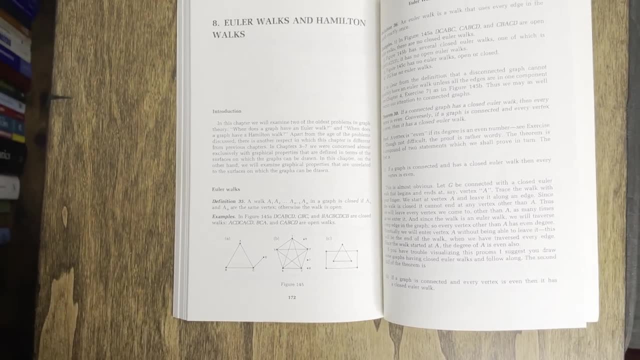 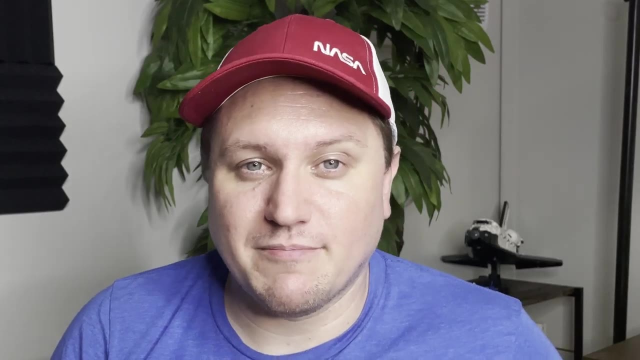 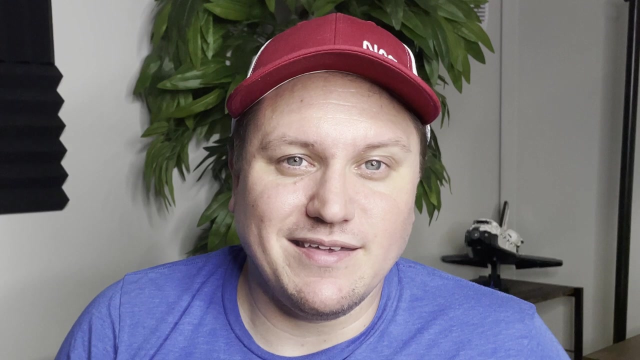 When Leonard Euler solved the seven bridges of conics, he was able to solve the first problem, which was the first problem, which was the first problem, which was the first expert problem. I've got a video on that as well And I use that problem to kick off my video series on doing graph theory with Python. 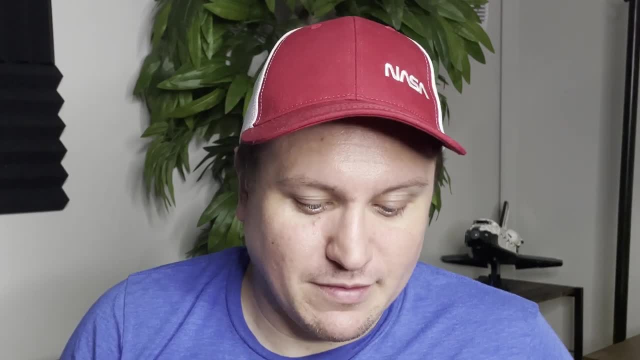 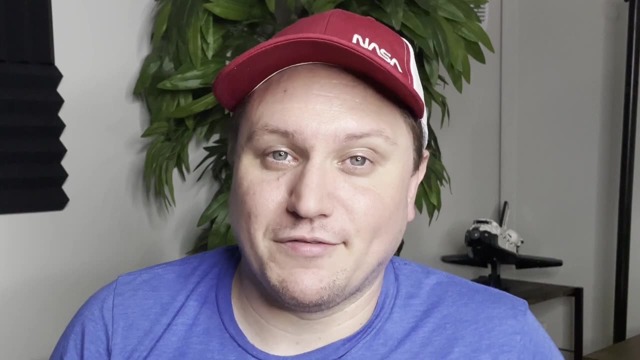 So I thought it was kind of interesting that we kind of approach things in a different order. I don't know, Reverse order is not the right word, but the topic that he saves for the last chapter is something that I decided to start my discussion of graph theory on. 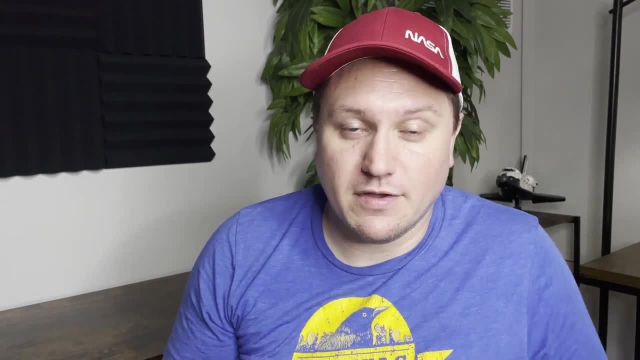 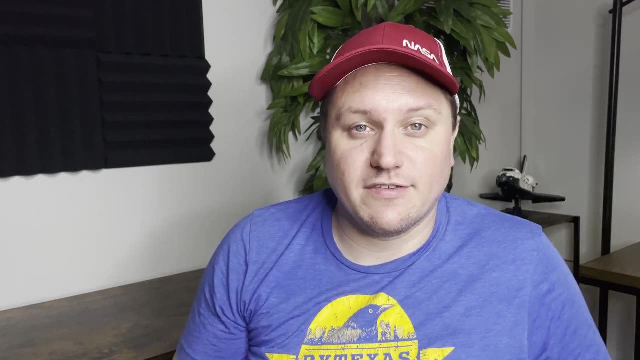 So that was kind of an interesting difference there. There's a wide range of topics in graph theory. If you read this book, you will have a good grasp of the kinds of things that graph theorists study and some of the approaches that they take. 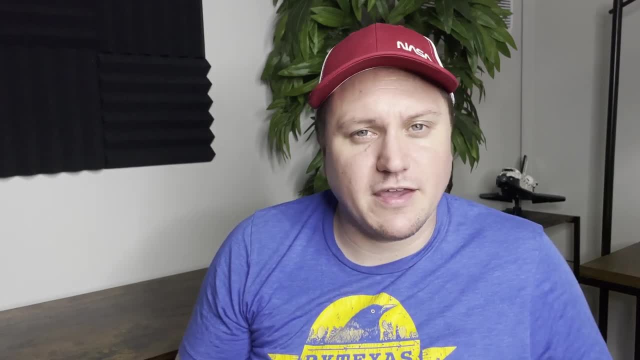 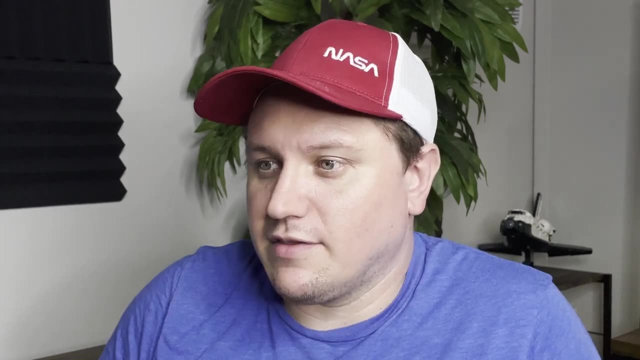 the techniques that they use and how they tend to think about problems. So I want to talk about some of the things that I really like about this book and why I consider it even one of my favorite math books of all time, And it really, I think, boils down to: 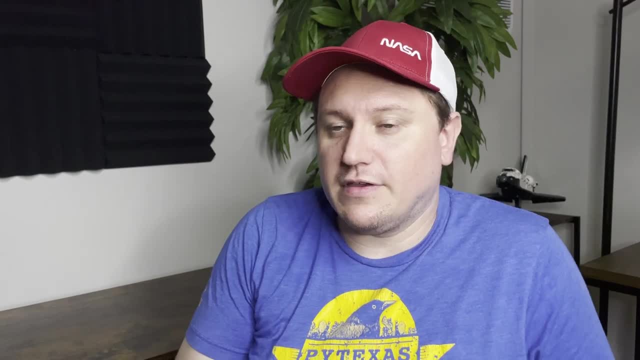 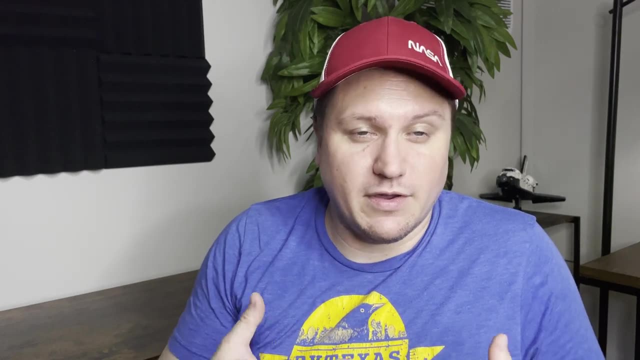 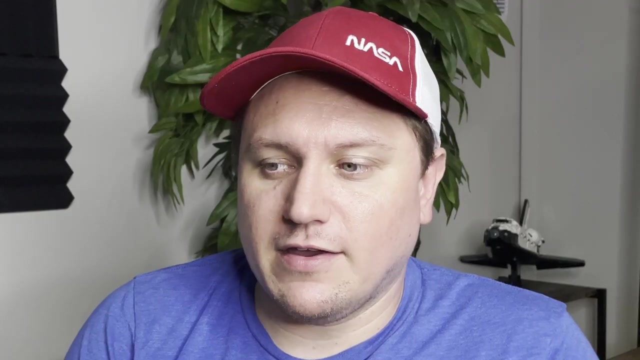 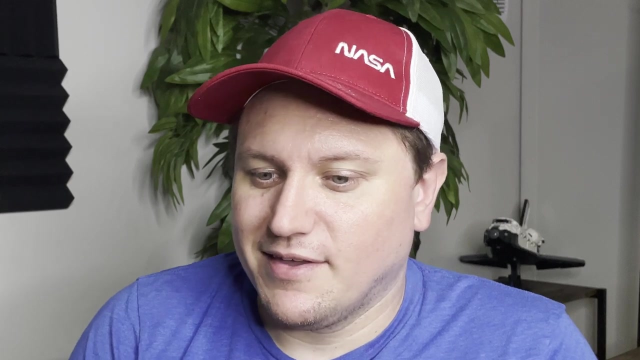 About four things. So the first is that the book is extremely approachable. Like I said, he wrote this in with a very general, very wide audience in mind And he really pulls it off. It's very, very gentle on the reader without sacrificing a lot of depth, which, again as a as a writer- when I see that I it's- it's just really amazing to see how well 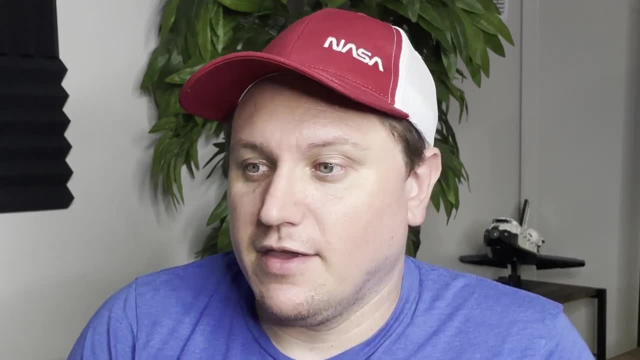 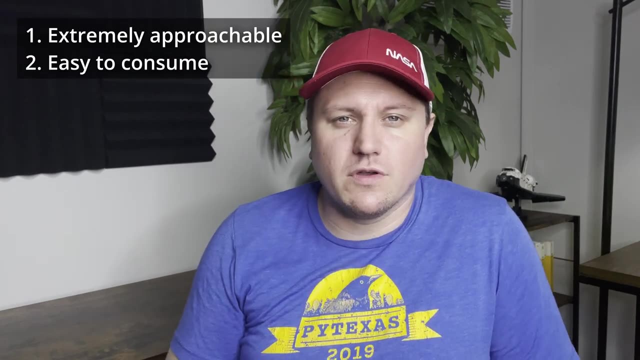 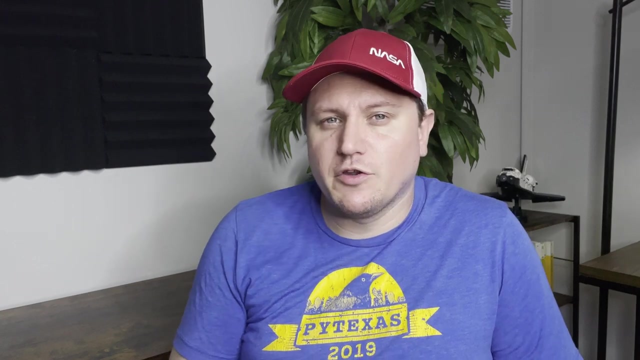 He's able to to pull that off. So the second thing that I really like about the book is that it's easy to consume. The chapters are relatively short. You can read most of them in probably 20 to 30 minutes. If you don't do the exercises, the exercises might take you a little bit more time than that. 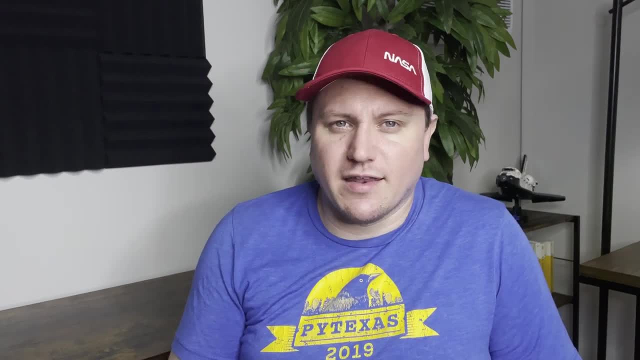 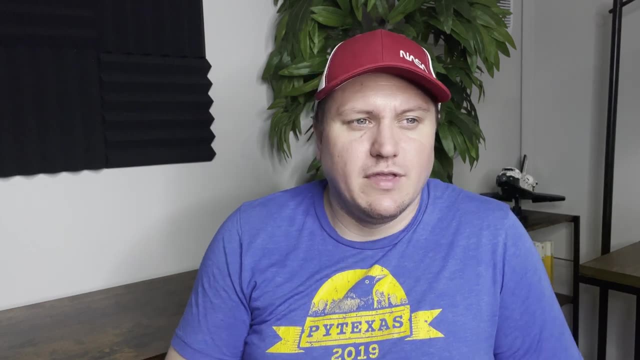 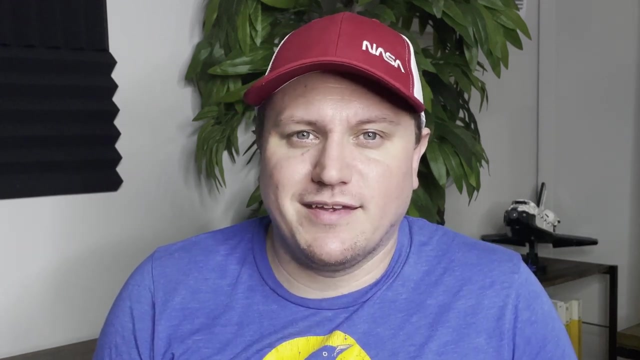 But just reading the chapters is not a huge commitment And once you've read the book two or three times, you can kind of pick and choose the chapters at will. And to this day I still will occasionally just pick it up, kind of flip to a random chapter or something that is on my mind. 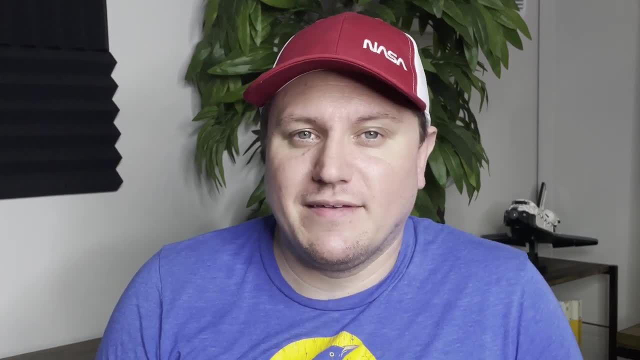 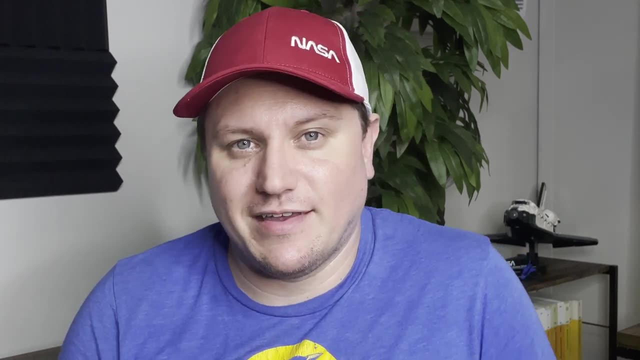 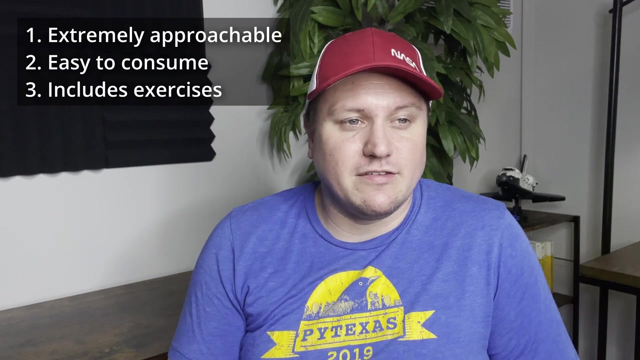 Sounds interesting And read that chapter and just re reengage with Trudeau's exposition and his thoughts on a particular topic in graph theory. The third reason that I really like the book is that it does include a number of exercises and that you know if you pick up any mathematics text. 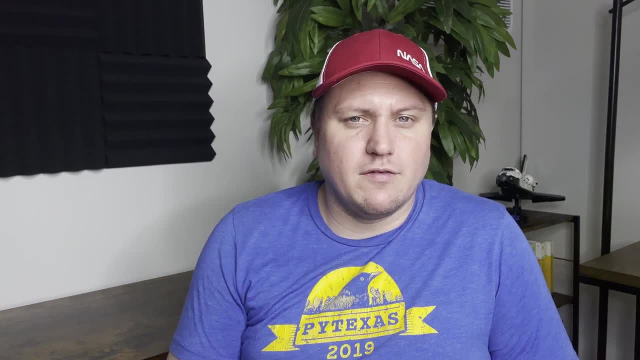 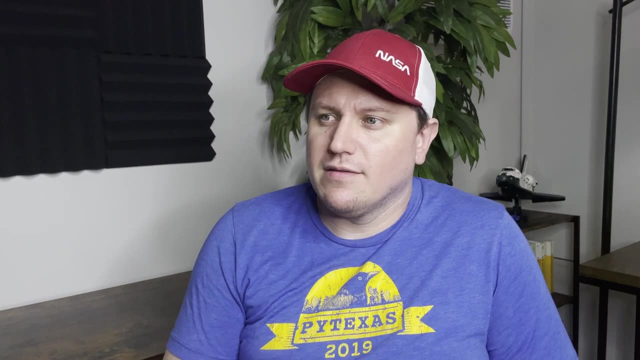 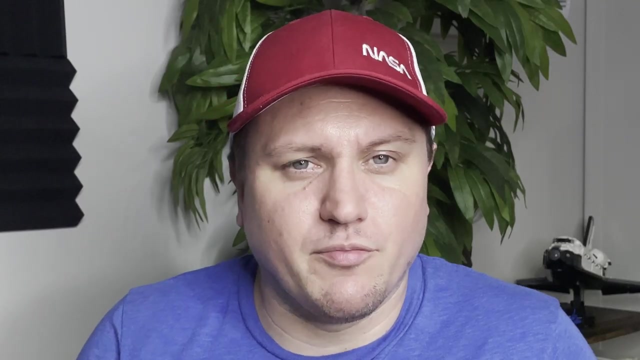 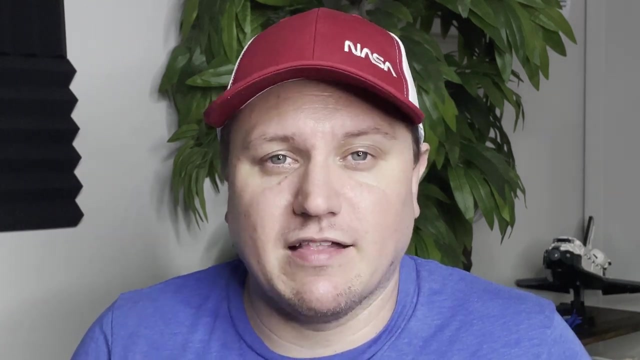 book. there's going to be lots of exercises in it, But a lot of layman's books don't have exercises, And this book is kind of teetering on the edge between being a layman's book and a mathematics textbook. The exercises, though, are approachable even to folks that don't have the pure mathematical background or haven't taken lots of advanced classes in mathematics. 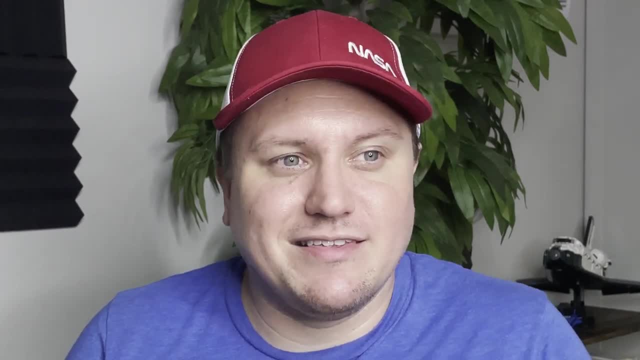 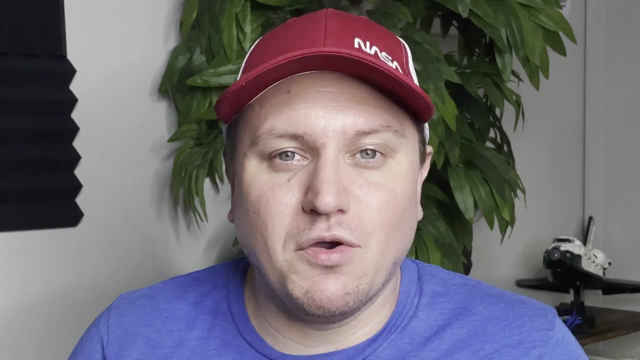 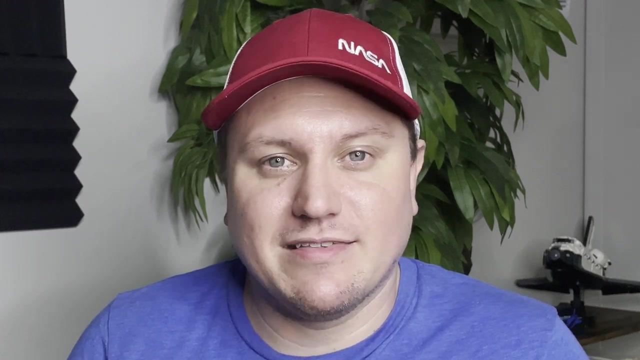 And I really, really like that. He doesn't Give you any indication of how challenging a an exercise might be, because you kind of go into it blindly And you might be surprised some of the things that you're able to solve just by reading about the different techniques that are used in the book. 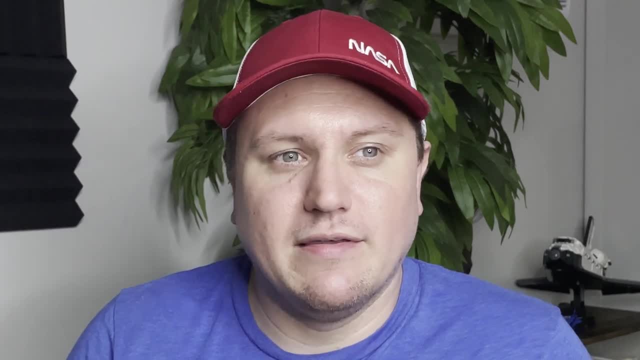 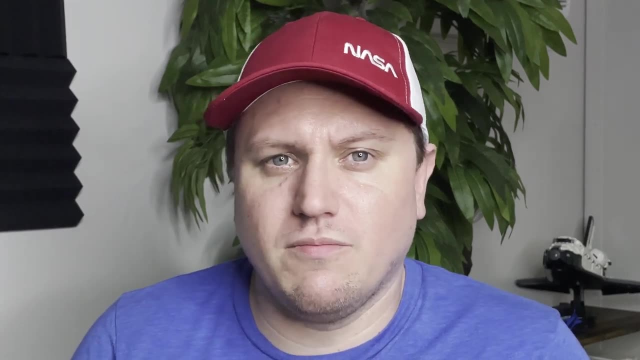 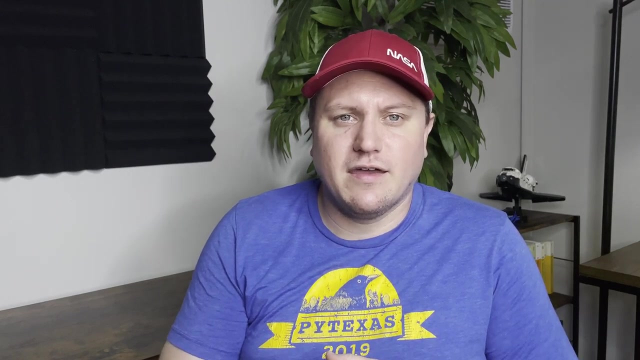 And on top of that it gives you a taste of what mathematical research kind of is, which is really neat. You don't necessarily always know how difficult a research problem is going to be. You don't know if, if you even know, If, if you even have the skills or the techniques ready at your hand to solve a problem. 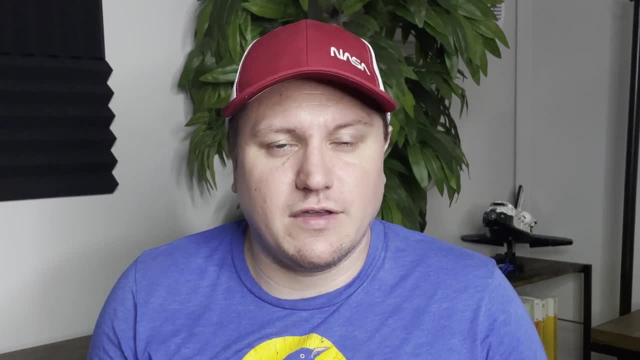 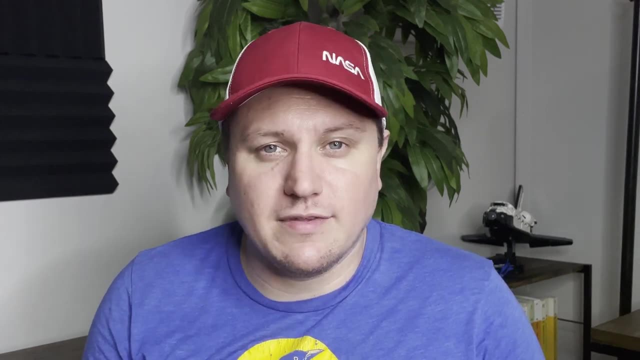 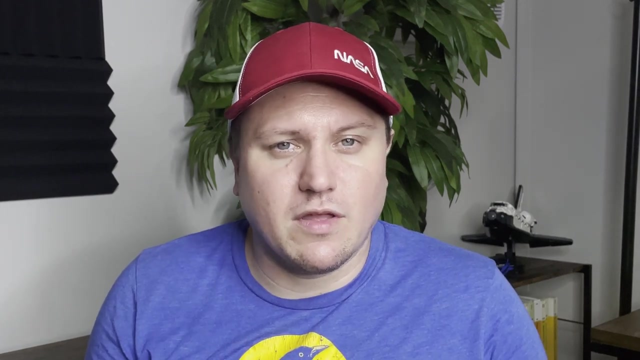 And the act of just thinking about a problem can often teach you things about yourself, about about mathematics- You can learn new things, You can invent new techniques. So just just engaging with an exercise, even if you you don't solve it as quickly as you might hope, or maybe even never solve it, 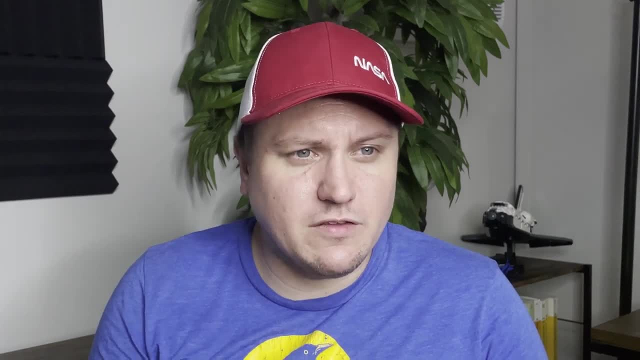 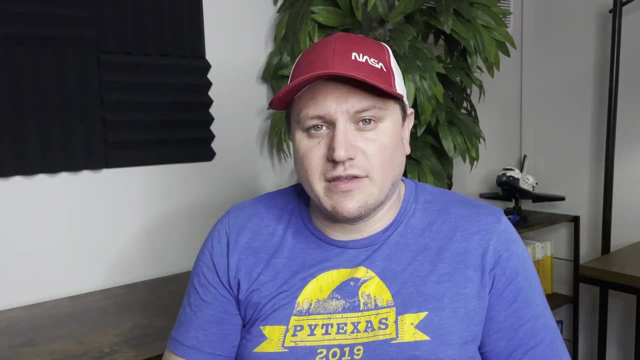 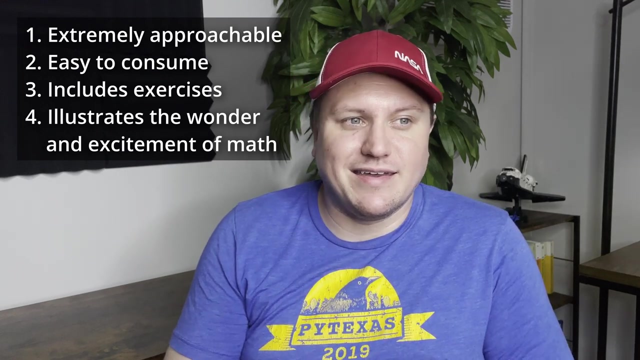 That act of engaging with it is going to teach you something about mathematics and about doing mathematics. Finally, the fourth reason that I really like the book is that it just does a really wonderful job of illustrating the wonder and excitement that doing mathematics entails and makes that approachable to a wide audience. 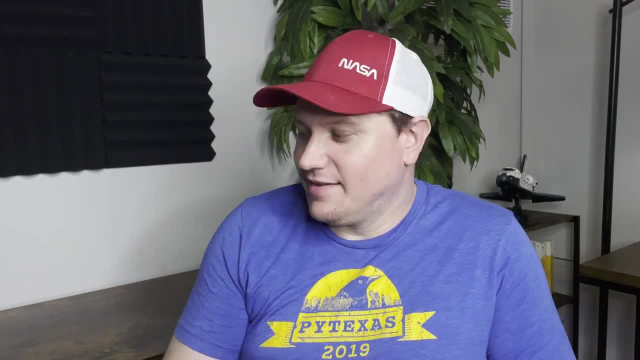 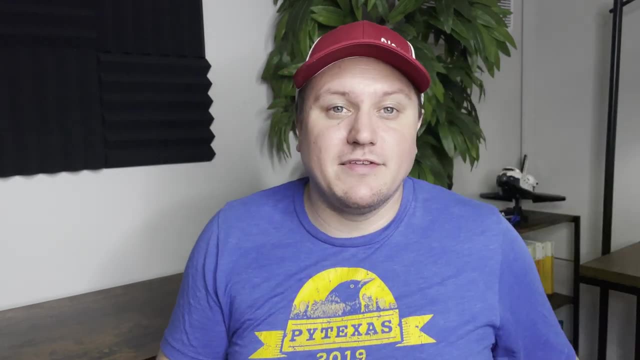 So those are the four reasons I like the book. Again, it is an introduction to graph theory by Richard Trudeau. If, if you read it, I would love to hear what you think about it. Did you enjoy it? Did you not like it? 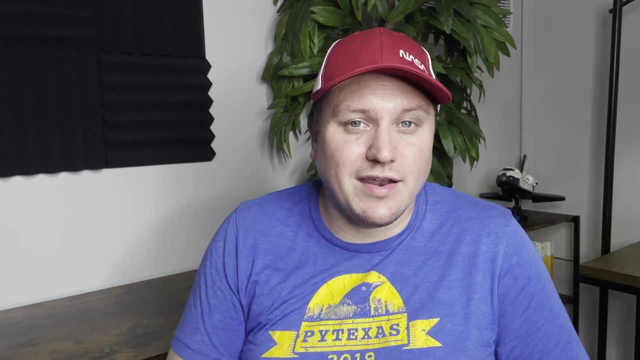 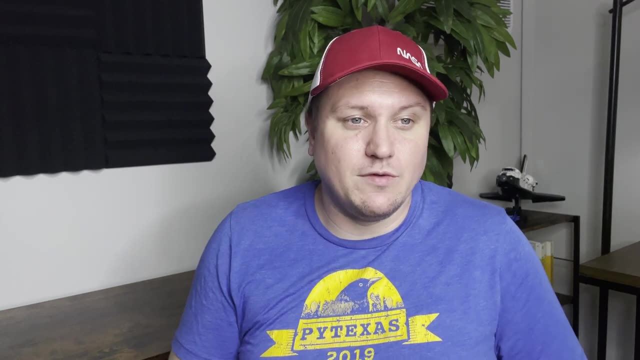 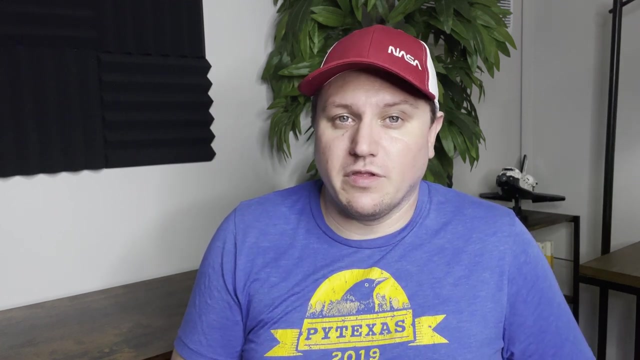 Let me know down in the comments If you have not read it. like I said, it's one of my favorite math books of all time. I highly recommend you get it. If you've seen some of my other content, you enjoy graph theory and the things that I've talked about on my channel, then I think you'll really enjoy this book. 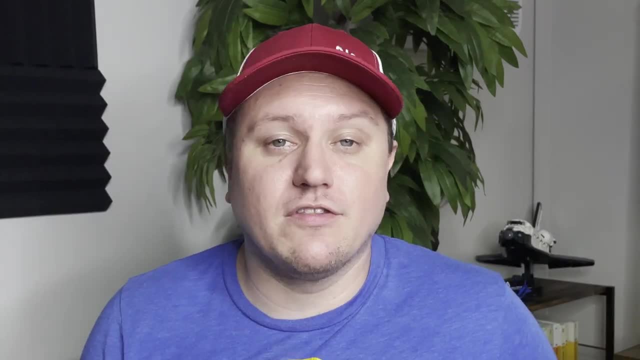 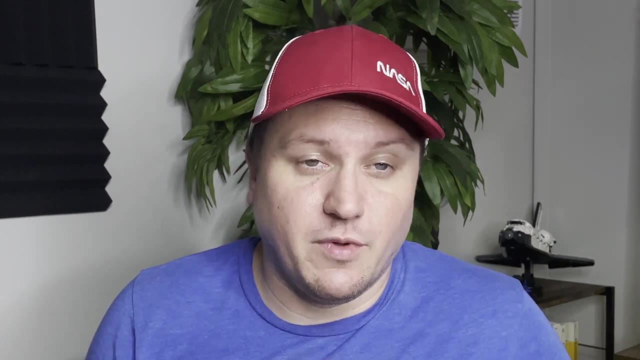 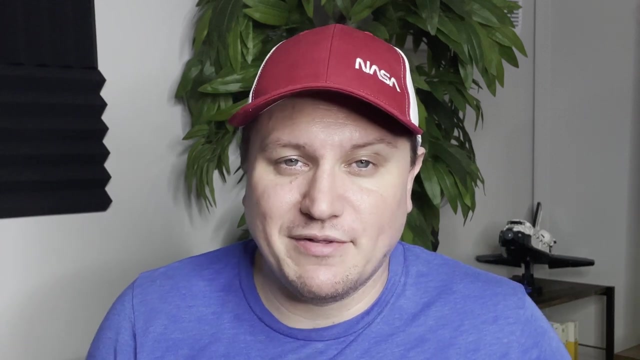 So I'll drop a link to to the purchase the book online. Purchase the book on Amazon down in the description. It is an affiliate link, so I will earn a little bit of small commission from it If you do end up purchasing. it just goes to help me keep running this channel and provide new and hopefully interesting content for all of you folks out there listening and watching.